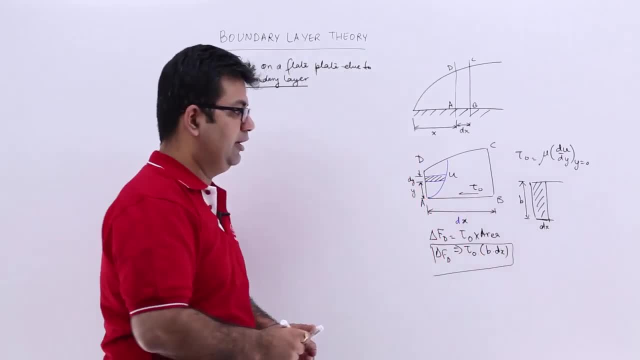 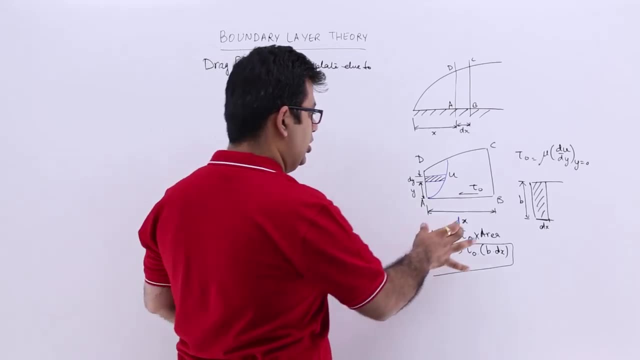 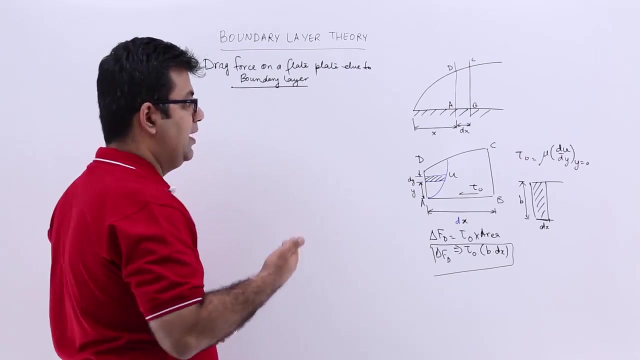 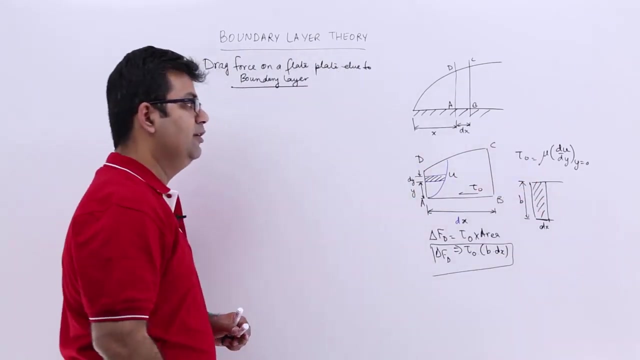 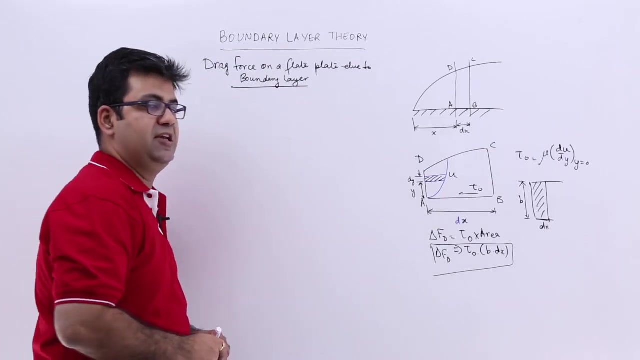 Okay, so we will have tau not into b, into dx, That is your delta fd. Now, this delta fd, or the drag force over this small element dx, should be equal to the rate of change of momentum over x or over delta x. Okay, so for that, let us find out the mass flow rate in phase ad and then we will find out the mass flow rate out of the phase bc. So for that, we have taken a small strip at distance y and the height of the strip is dy. So this delta fd, or the drag force over this small element dx, should be equal to the rate of change of momentum over x or over delta x. Okay, so for that, let us find out the mass flow rate in phase ad and then we will find out the mass flow rate out of the phase bc. So for that, we have taken a small strip at distance y and the height of the strip is dy. So for that, we have taken a small strip at distance y and the height of the strip is dy. So for that, we have taken a small strip at distance y and the height of the strip is dy. So for that, we have taken a small strip at distance. 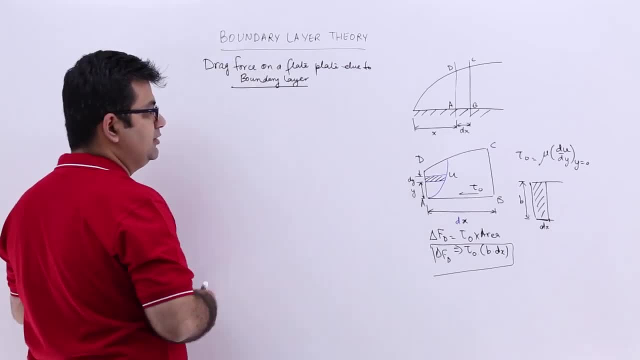 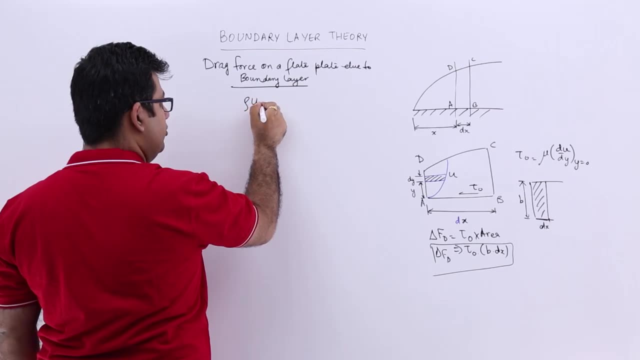 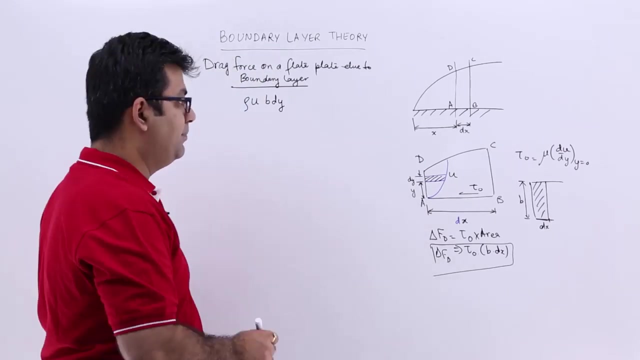 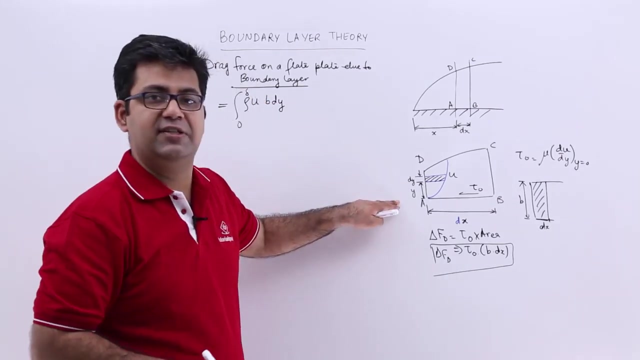 so through this strip the mass flowing is density into velocity, into area, so you will have rho into u, into b dy. this is the mass flow rate. through this you can say strip. so if i integrate it from 0 to delta you get the mass flow rate in through phase ad. 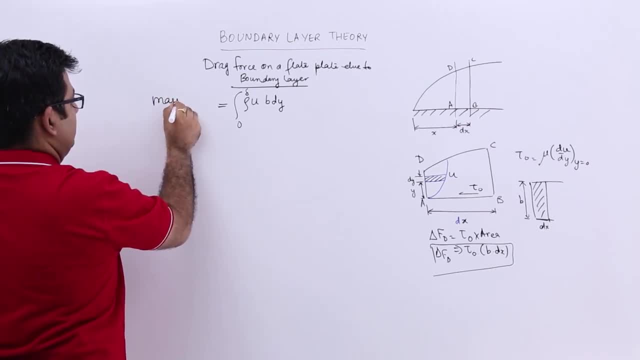 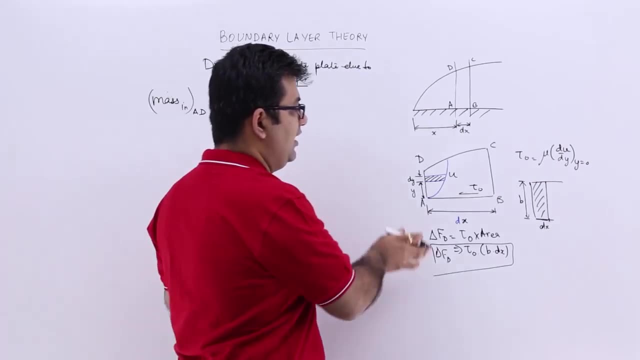 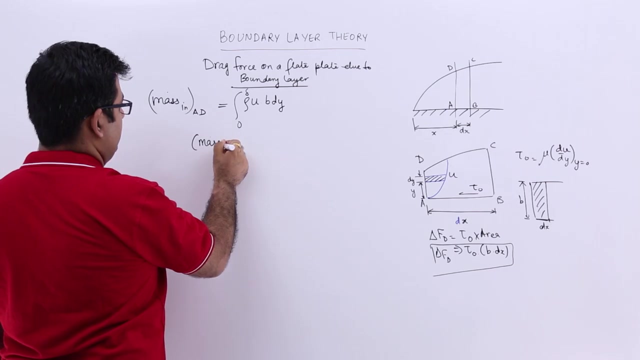 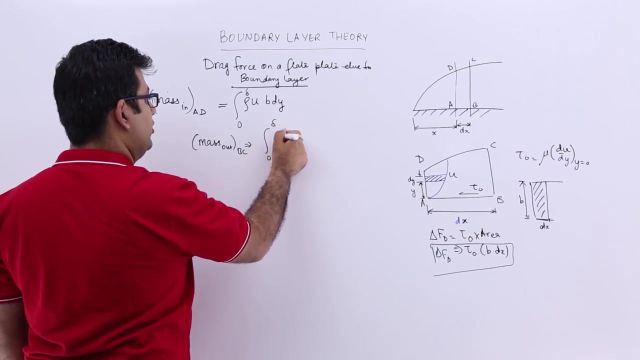 so this is mass dot in and this is from phase ad. now there is some mass which is leaving the phase bc, is that right? so that will be equal to mass out and this is phase bc. so you will have this rho into u, into b dy plus. 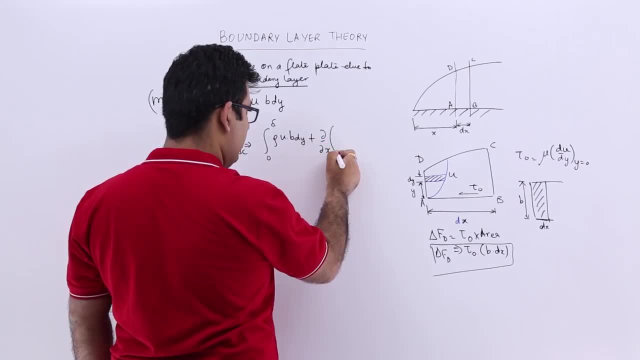 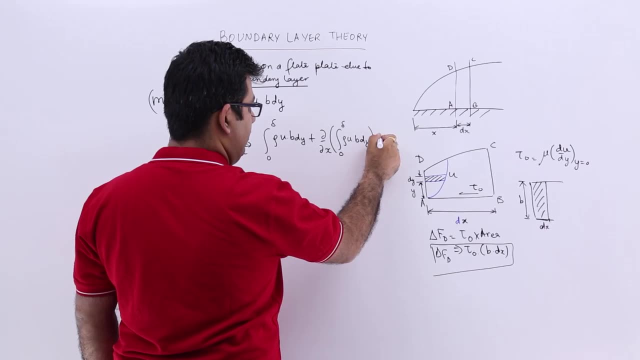 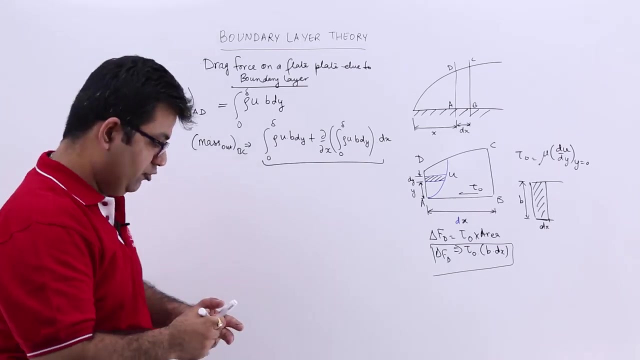 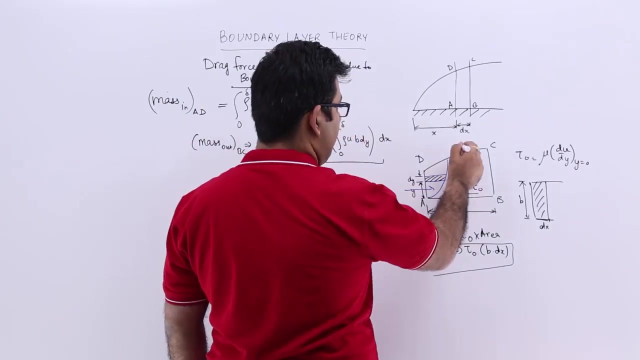 curly y by curly x of integral 0 to delta rho u, b, dy into dx. so that is the mass which is leaving the phase bc. now, if you apply the continuity equation of the conservation of mass, you have mass coming in from this. you have mass coming in from this. 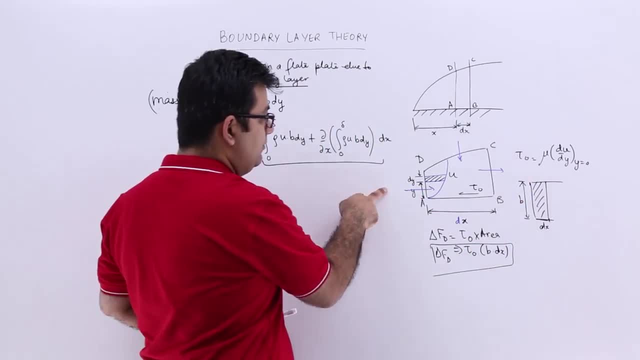 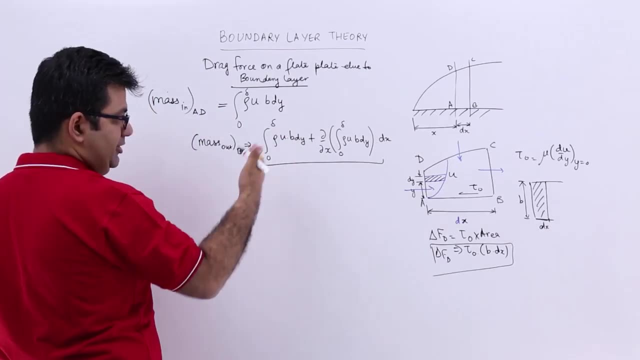 and you have mass leaving bc. so this mass in plus this mass in is equal to that mass out. so you will have mass in from ad plus mass in from dc is equal to mass out from bc. so to calculate the mass in from dc, so mass in from phase dc. 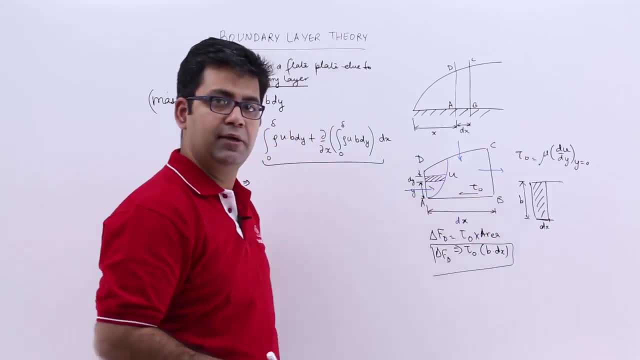 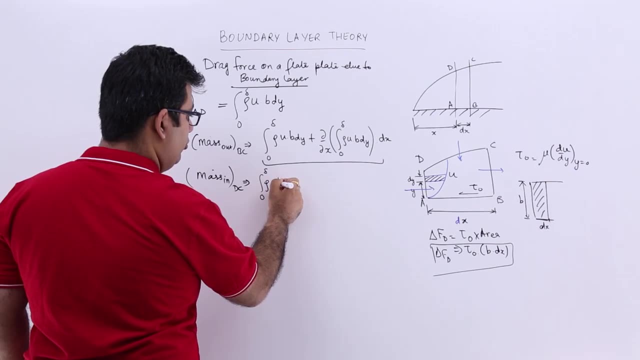 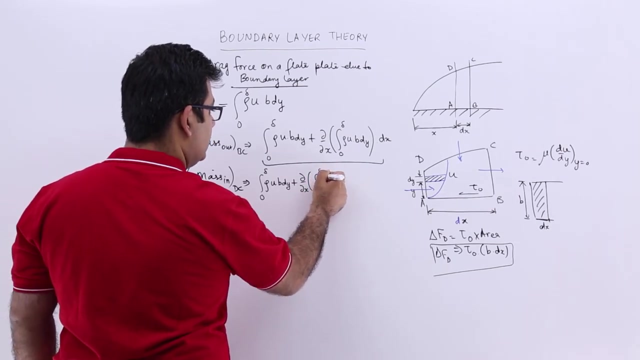 is equal to mass out of bc. that is this entire expression. ok, 0 to delta rho u into b dy plus 0 to delta rho u into b dy plus 0 to delta rho u into b dy plus 0 to delta rho u into b d y into dx. 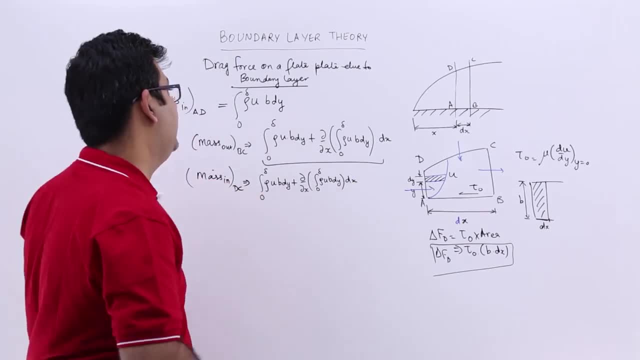 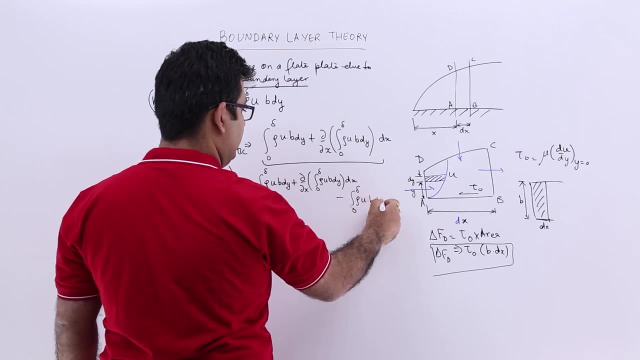 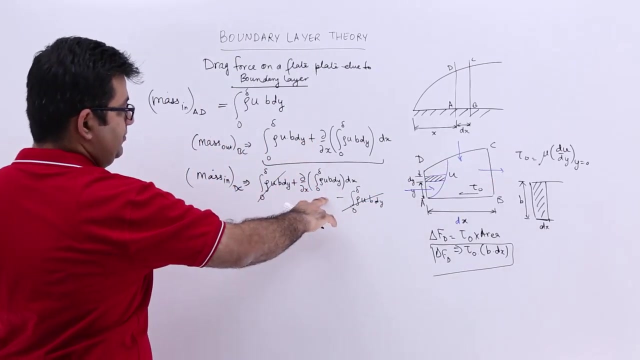 ok, minus the mass coming in from this ad, so that is this part. so minus integral 0 to delta rho u, b, d, y, so you can strike off this. so the mass which is coming in from this phase dc is this part, so you can rewrite it. 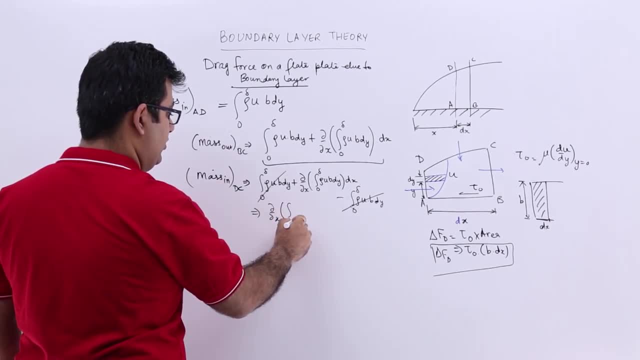 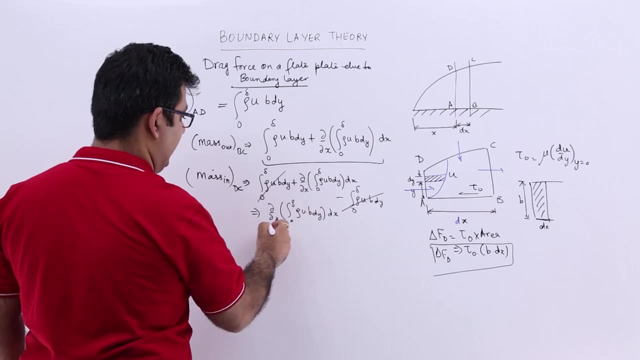 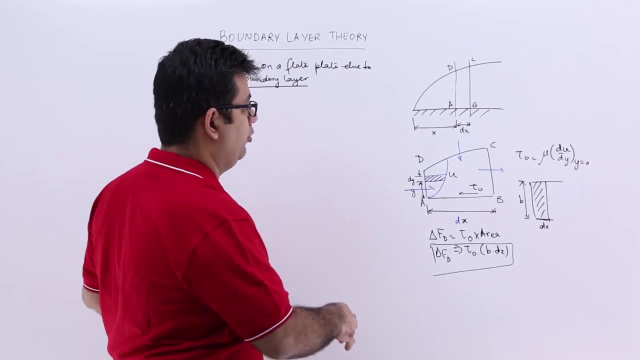 it will be rho Curly by curly, x of 0 to delta rho uv dy into dx. That is the mass coming from phase dc. Now we have seen the mass flow in and mass flow out and then mass flow in from dc as well. 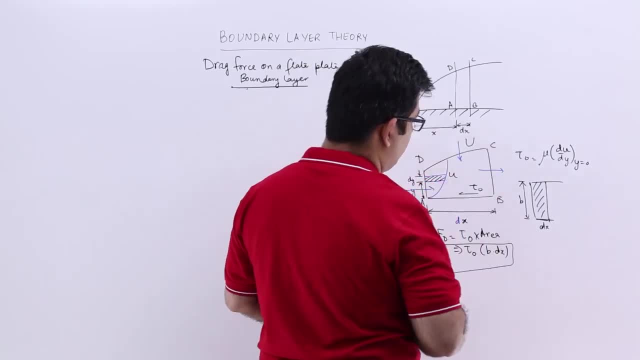 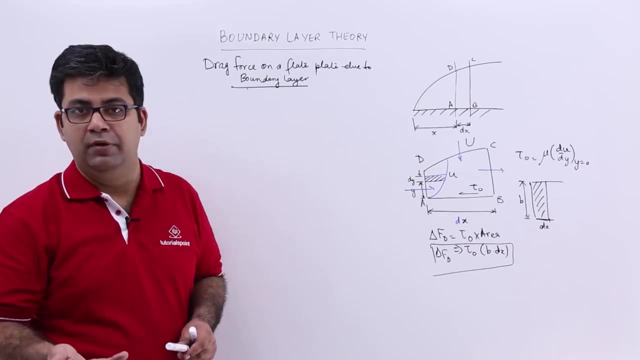 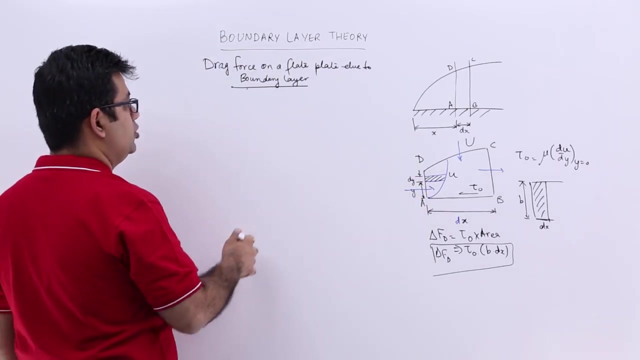 Now the mass flow in from dc is at a constant velocity, capital U that is equal to the free frame velocity. okay, Now we look at the momentum flow per second. So if you talk about the momentum flow in through the phase ad, so it will be rho into u, into bd y. that is the mass. 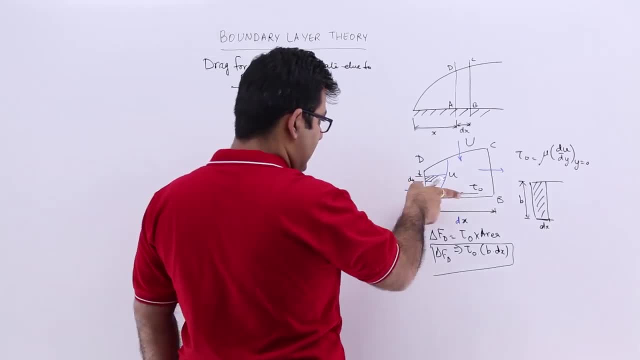 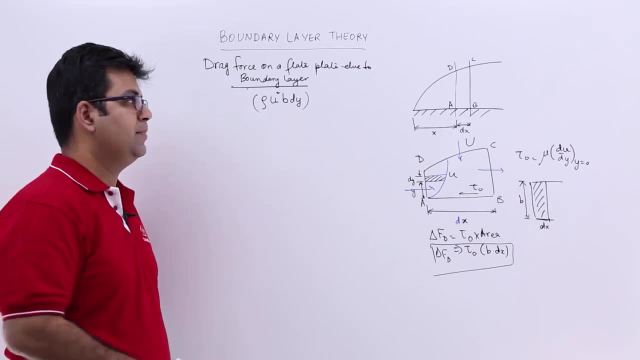 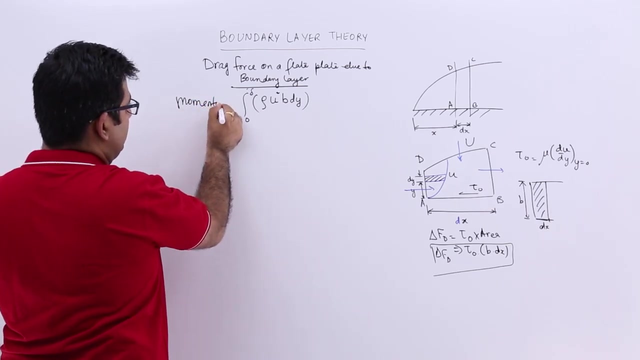 And if you multiply this with the velocity, because through phase ad the velocity is small u only, So you will be getting a square of the velocity. And if you integrate this, This is, This is the momentum, This is the momentum in through phase ad. 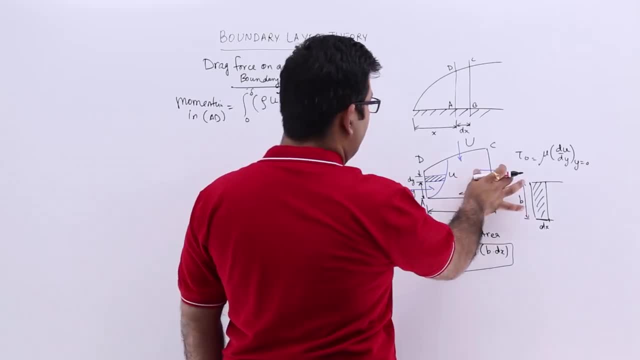 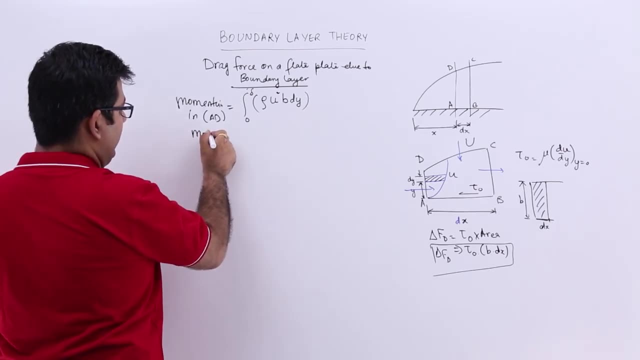 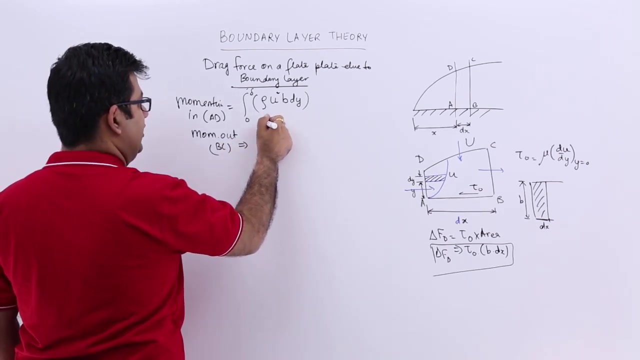 Okay, Then there will be some momentum which will be going outside the control volume from phase bc, So that would be momentum out from side bc. That will be 0 upon delta. Again, it is going out at a velocity u, So you will have small u square only. 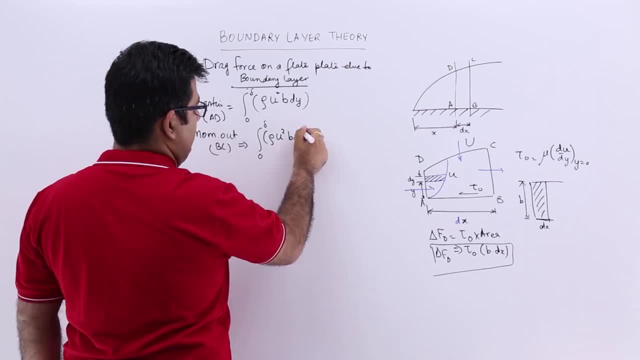 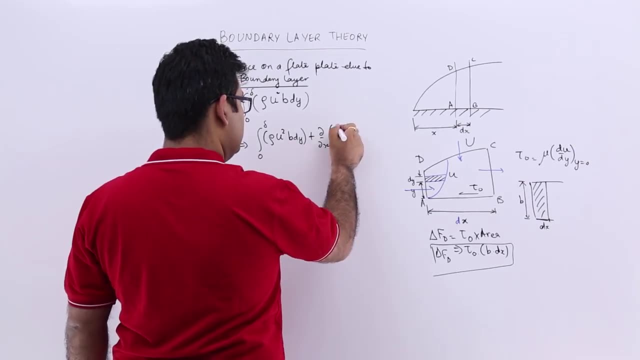 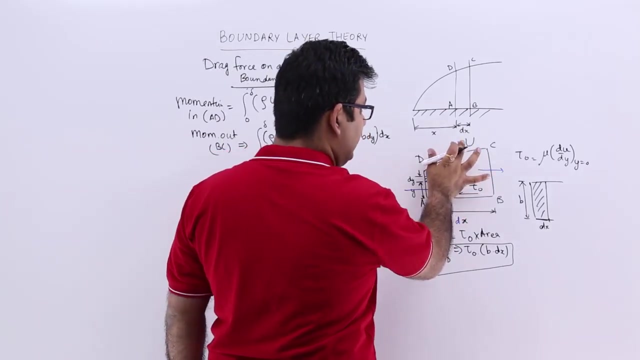 So it will be this plus curly by curly x, Curly by curly x into 0 to delta. rho u square bdy into dx. Alright, So this is what you get. Then you have some momentum coming in at this velocity from the side dc. 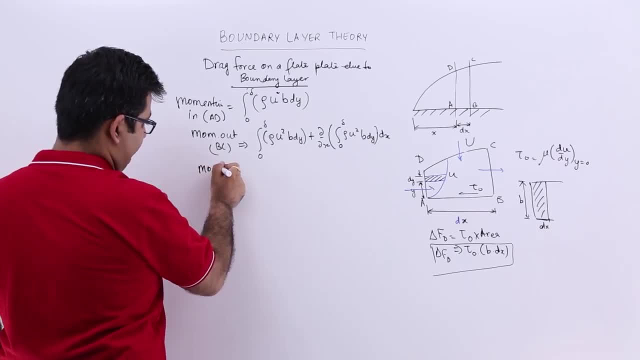 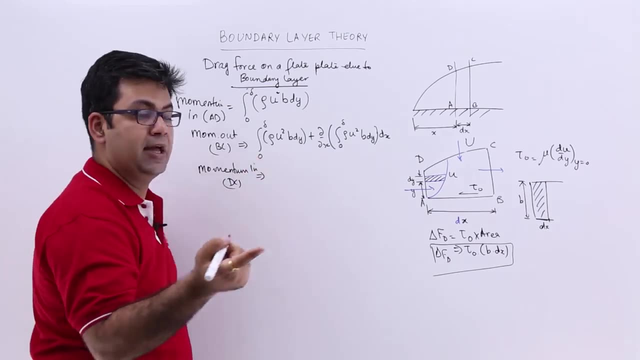 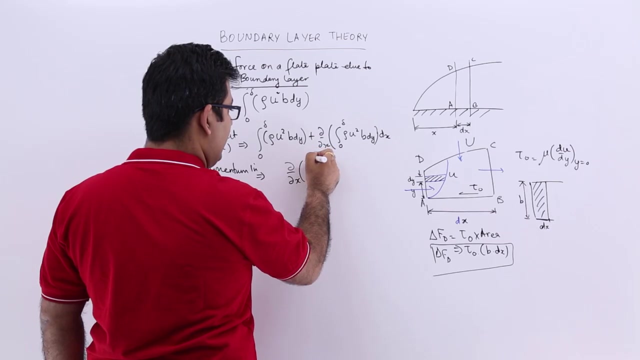 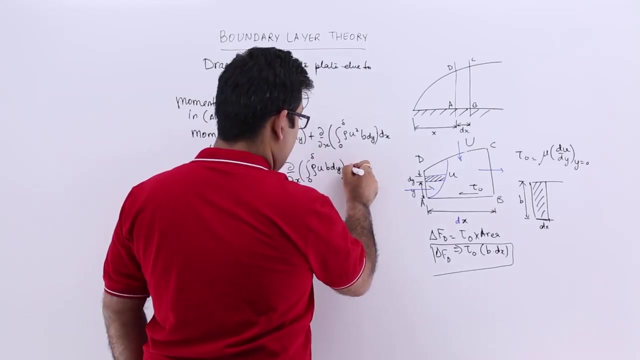 Now, momentum in from dc. Now we know that the mass coming in from dc was this much That is curly by curly, x of integral 0 to delta, rho into u, into bdy, into dx. Okay, Now the velocity of the flow coming in is capital u. 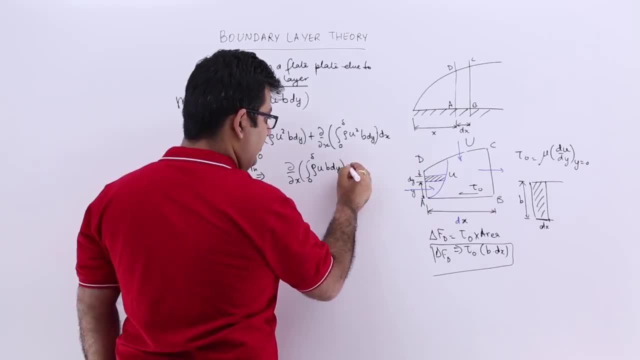 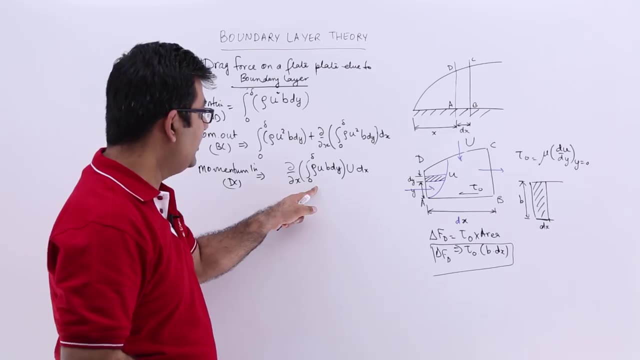 So I will have to multiply. So I will have to multiply this with capital u and then write dx. So this is small u which comes from this expression, And you multiply this mass with the velocity at which the flow is coming in. 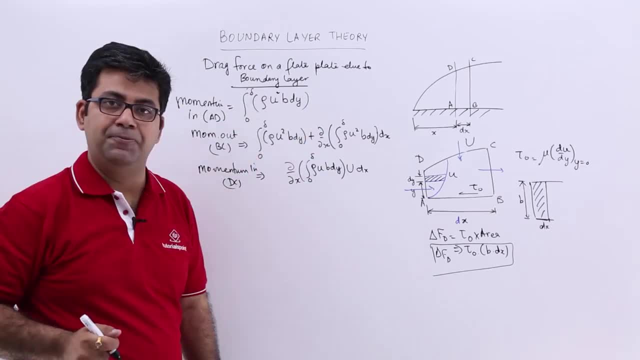 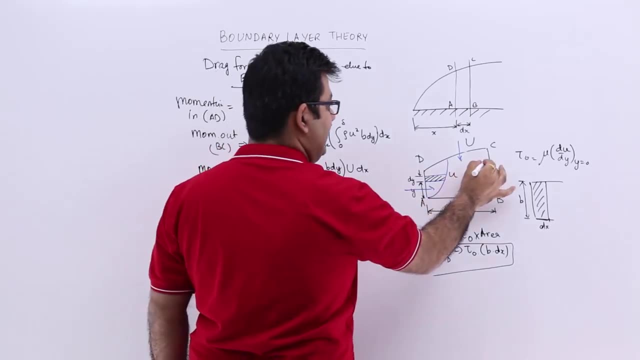 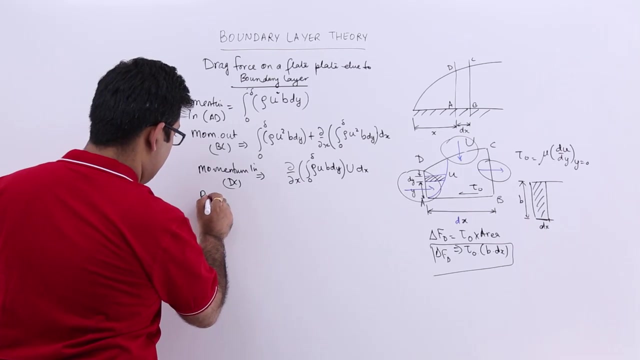 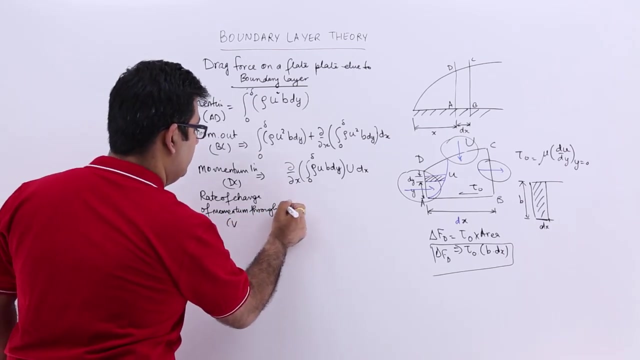 That is capital u to get the momentum coming in from phase dc. So the rate of change of momentum through this control volume would be this minus this, minus this. Okay, So you will have Rate of change of momentum through the control volume. 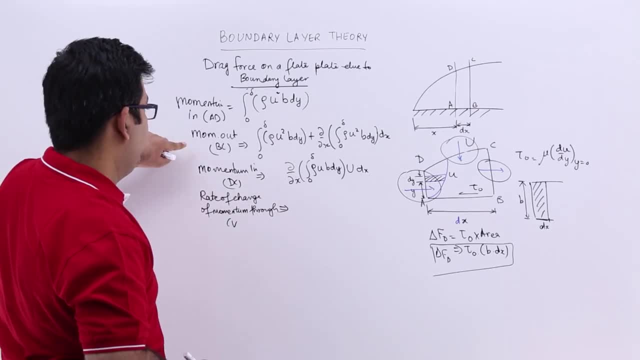 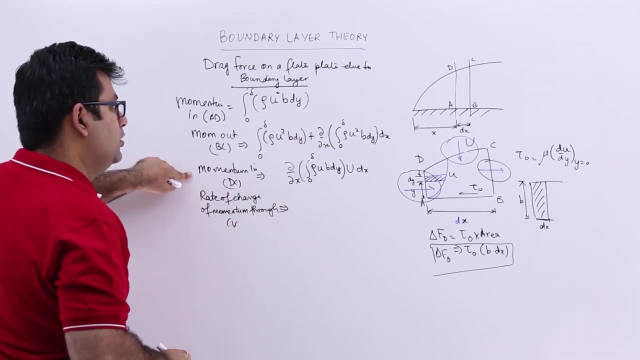 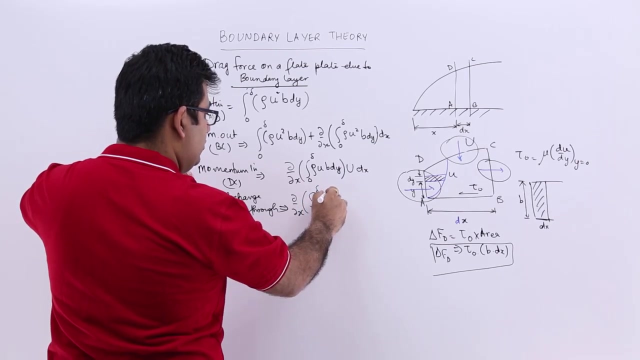 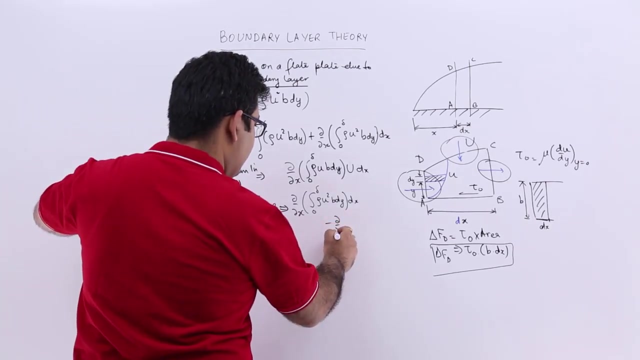 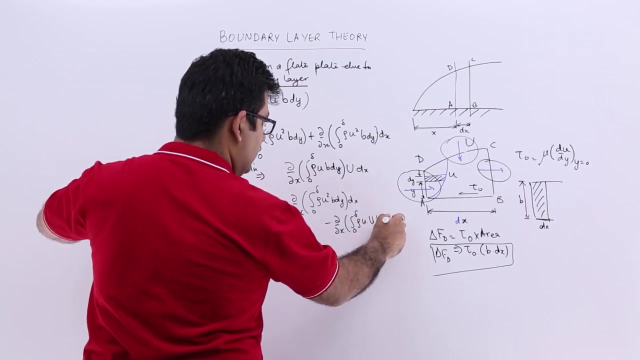 Okay, So bc is this bc minus ad minus dc. So you can subtract this part and that part, So it will be gone. So you will have curly by curly x, Okay, Of integral 0 to delta rho into u square bdy, dx. minus this momentum which is curly by curly x of integral 0 to delta rho into small u capital, u bdy into delta x for dx. 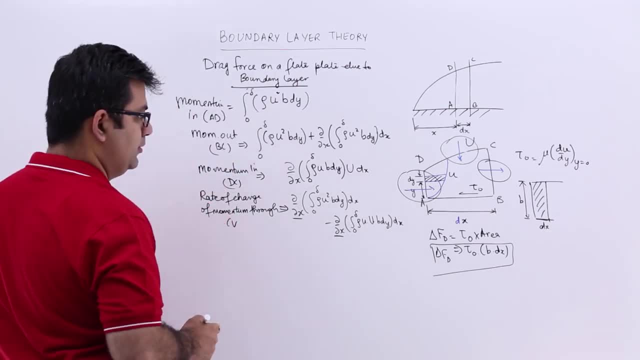 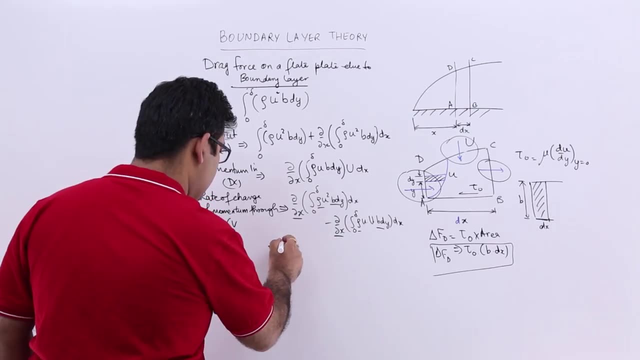 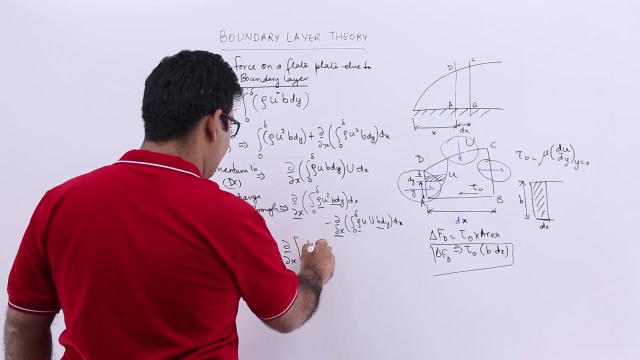 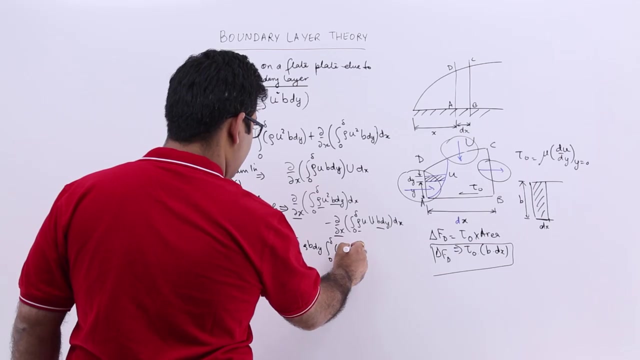 Okay, So let us take curly by curly x common and then we can take rho and bdy also common, Alright, So we will have curly by curly x of rho into bdy, into integral 0 to delta. We will have small u square minus this. 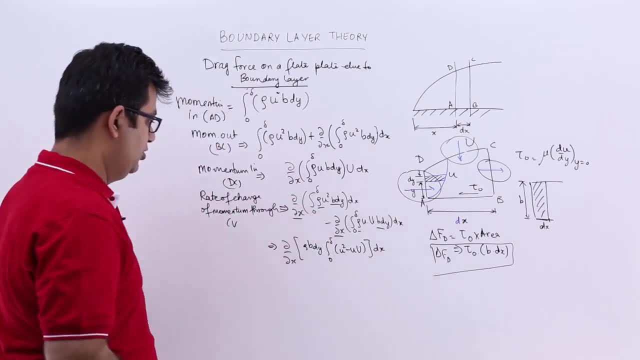 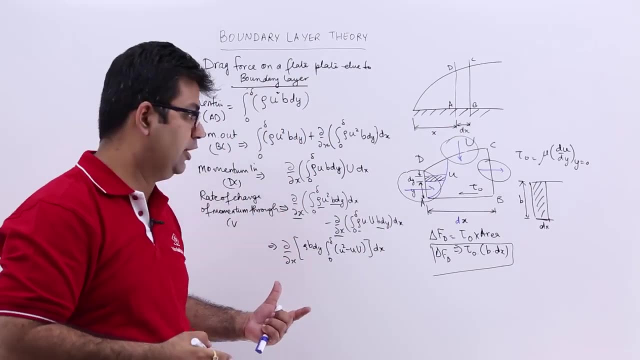 Okay, And then at the end you will have dx. So this is the rate of change of momentum through this control volume. Now this rate of change of momentum through the control volume Has to be equal to this drag force. Okay, 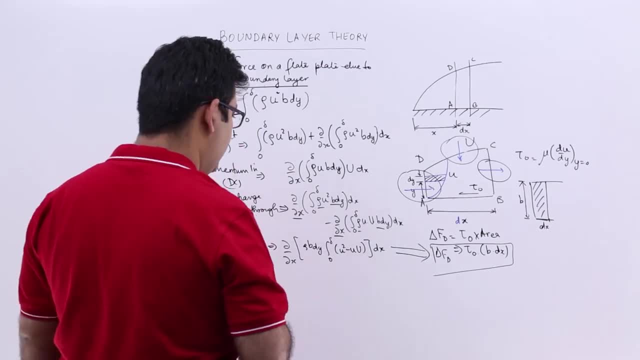 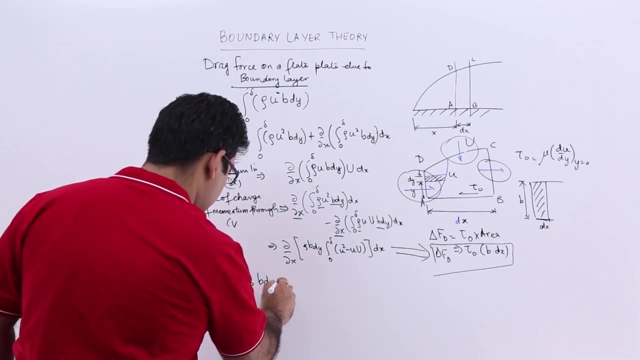 And because there is no external force which is active on it, You can write it down like this: So, minus tau, naught into bdx, This is equal to the rate of change of momentum. So you will have curly by curly, x into rho, into b, into 0 to delta. 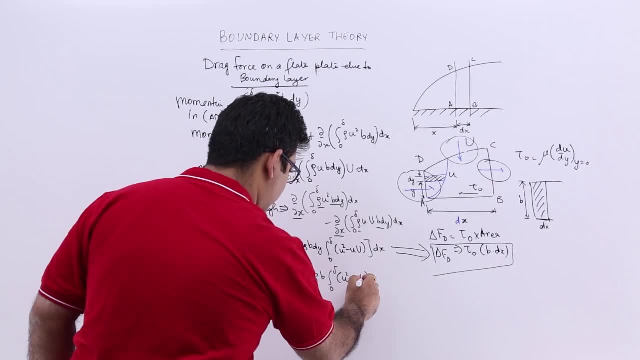 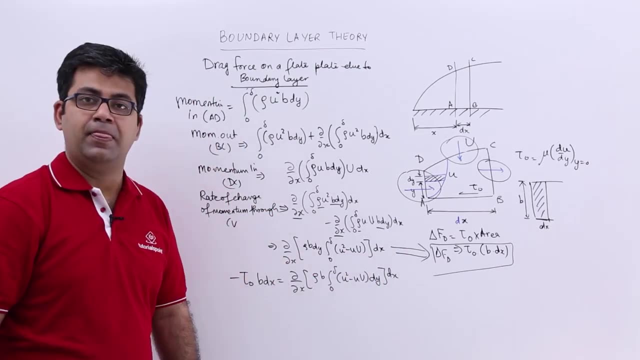 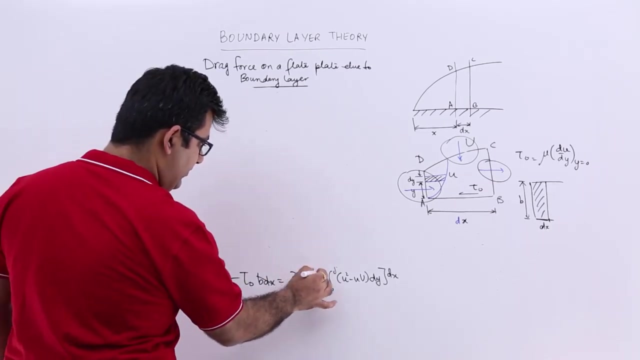 Then you will have small u square minus small u into capital, u dy Into dx. So this is what you will get. Okay, So let us explore this a bit. You can strike off bdx and bdx from the two sides. 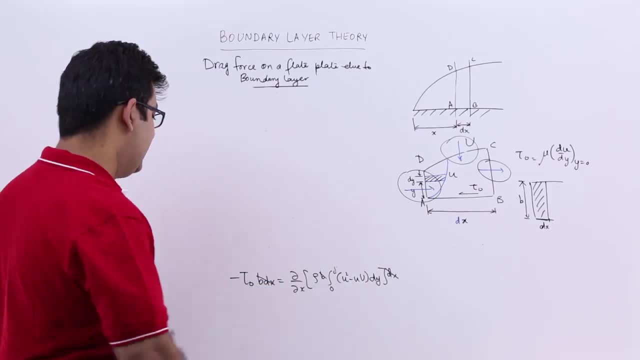 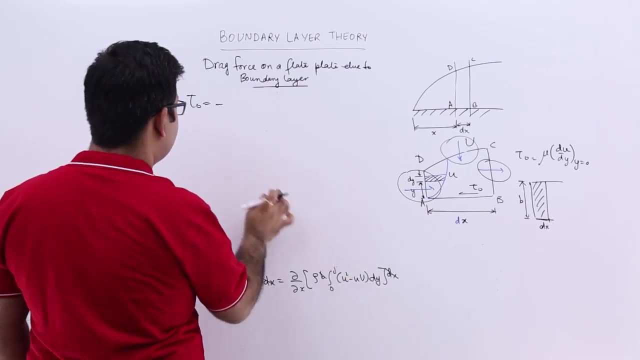 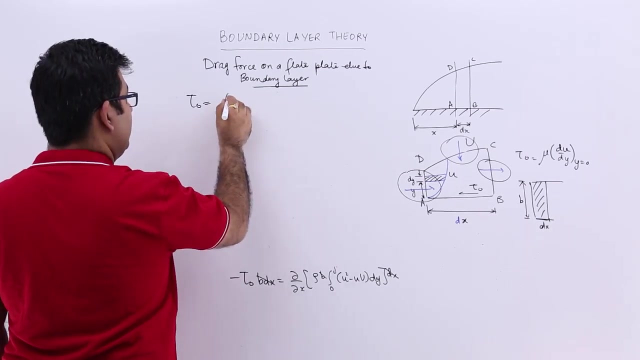 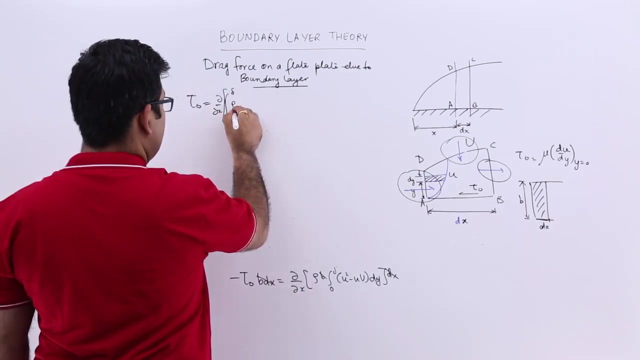 Let me take negative sign on to the other side. That will give you tau. naught is equal to minus, So let us get rid of the minus. And And. And And will have integral or curly, by curly x first into integral 0 to delta rho, then you will. 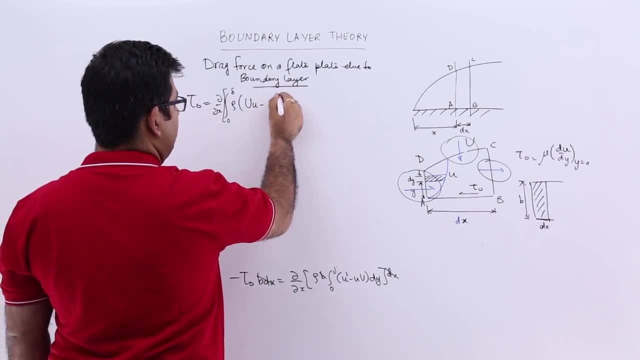 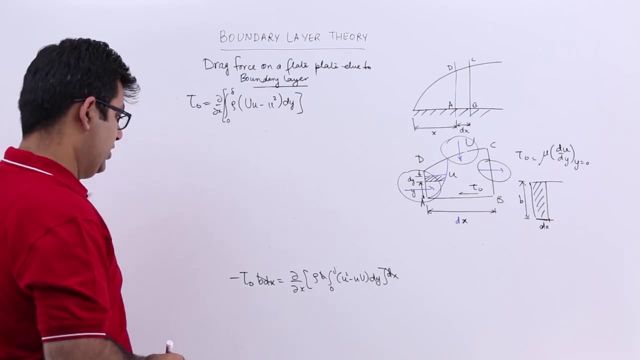 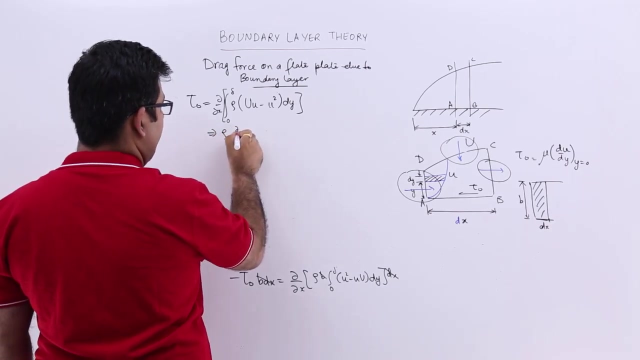 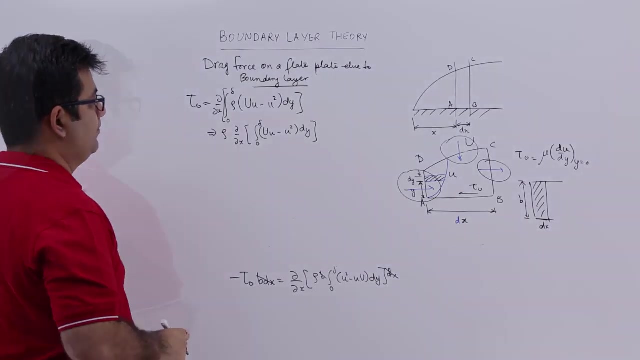 have u minus small u into this, into dy. this is what you get, okay, so let's get rho outside, because let's assume that the flow is incompressible. so you will have integral 0 to delta this minus small u square dy. let's, you know, alter it algebraically. so let's multiply and divide. 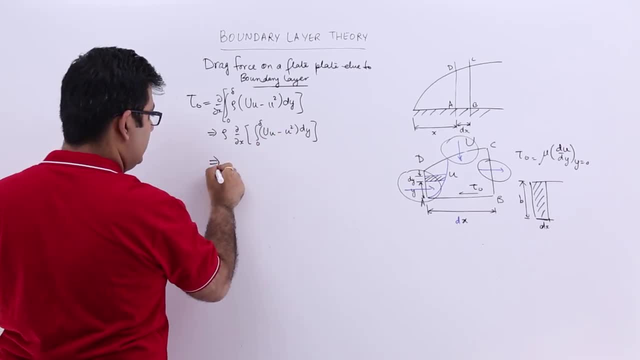 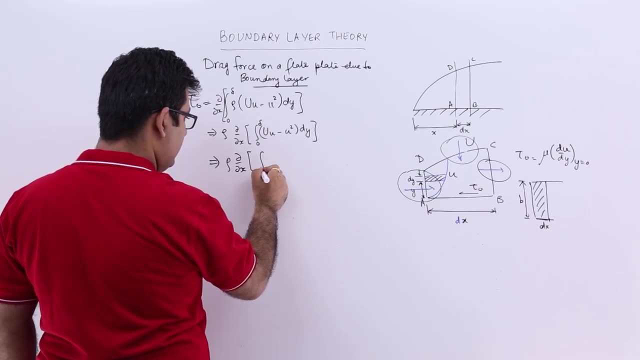 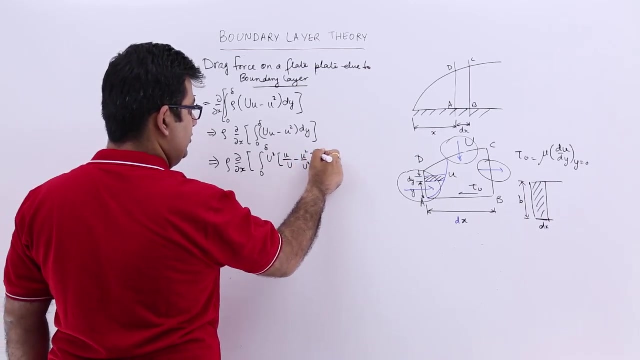 this expression by capital u square. so you will get rho curly by curly x into integral 0 to delta. let's multiply it by capital u square and you will have small u upon capital u minus small u square upon capital u square. so this would be the expression.